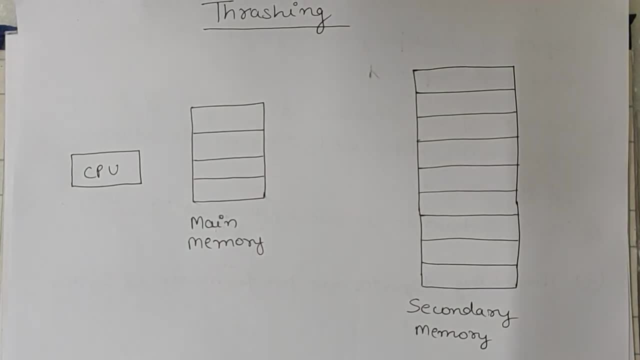 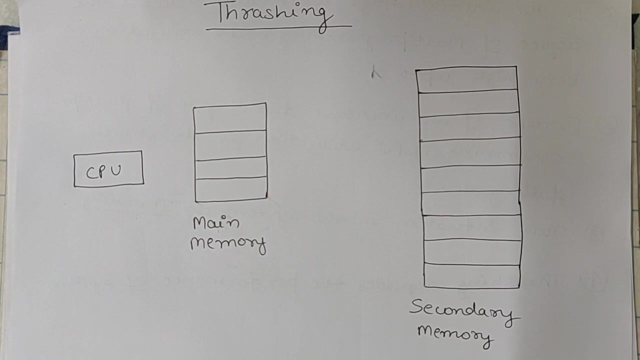 Hello everyone, welcome to operating system tutorial. In this tutorial I will discuss the concept of thrashing. This is the most important topic in operating system, in paging concept. basically, This is the very important concept. So please listen carefully what thrashing is Okay. so again, let's take an example. With the example we can easily understand. 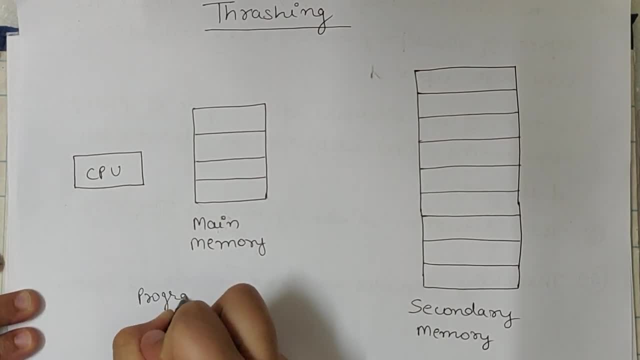 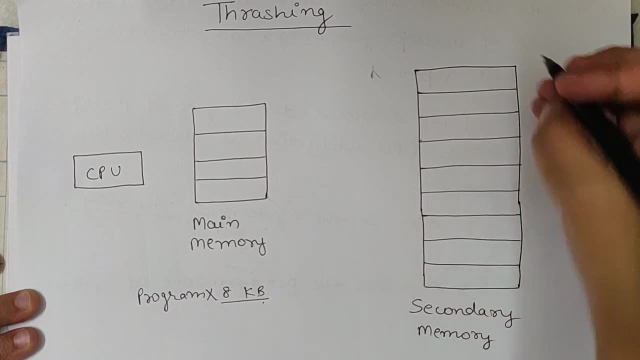 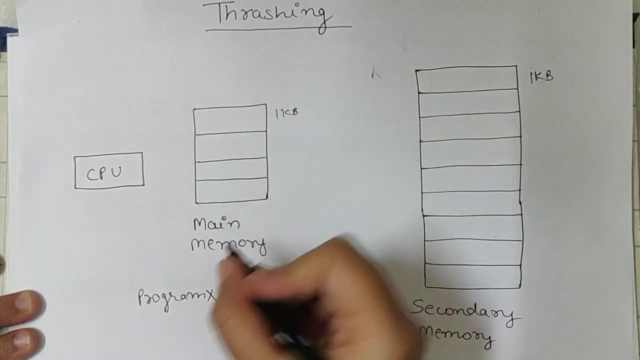 what thrashing is. Say suppose we have a program of size, program x, of size 8kb, Okay, and we divide this program into 8 pieces. This is secondary memory of size. each partition is of size 1kb. Similarly, 1kb is in main memory Equal size partition. we have done. 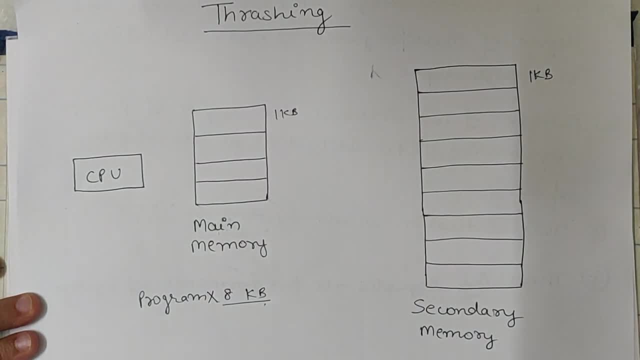 paging- Basically, thrashing is the concept of paging. Okay, so if you have not seen the videos of paging, so please go and watch the previous videos about paging. Okay, so let's start. So paging is done Here. we have done partitions: 1kb each partition. Similarly, 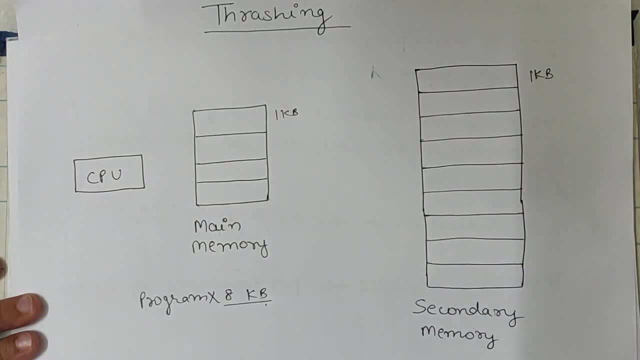 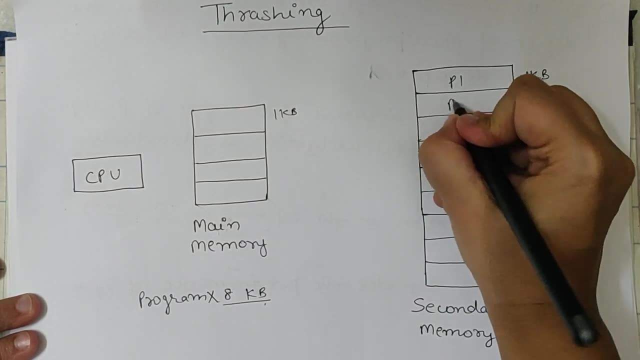 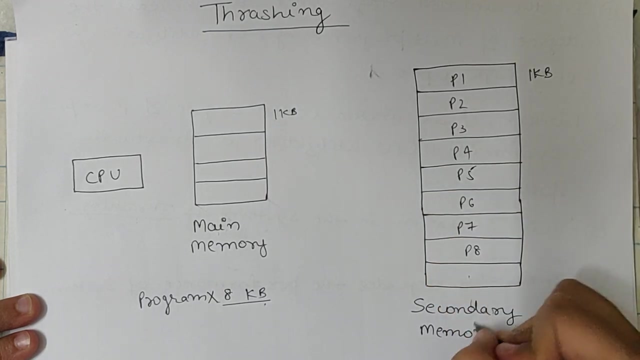 in main memory 1kb each partition And program x is loaded in secondary memory And program x is of size 8kb. Okay, so 8 pages are done: P1, P2, P3, P4, P5, P6, P7, P8.. Okay and so. 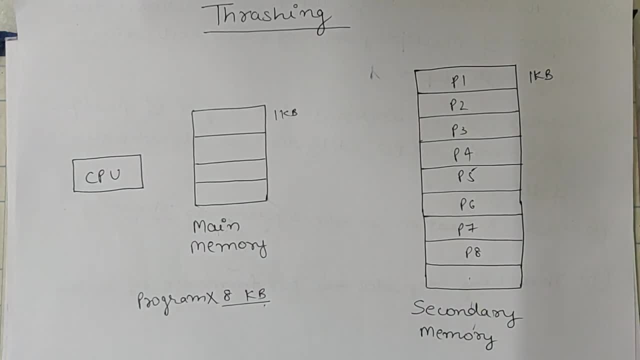 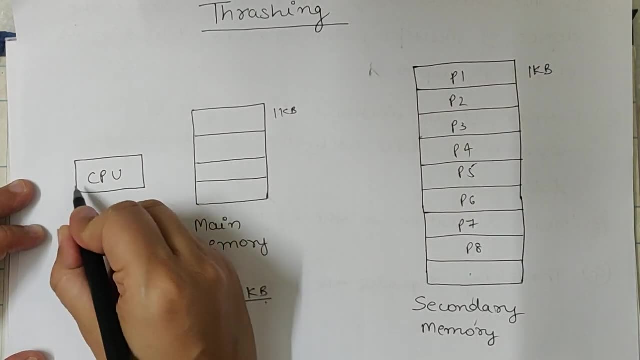 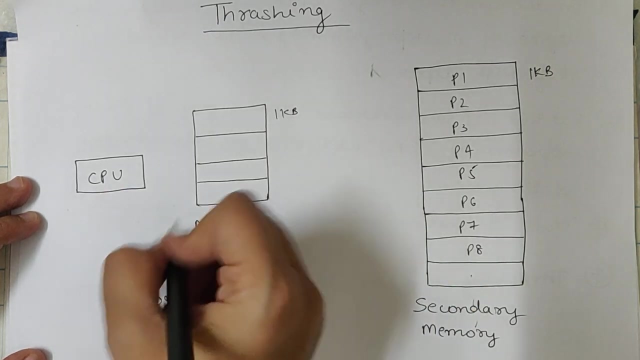 on. Now there will be pages of some other program. We mean program x. Okay, so now, right now, what happened is CPU started to demand Demand paging. I have already discussed So in the previous videos, So you can watch my previous video about demand paging. So 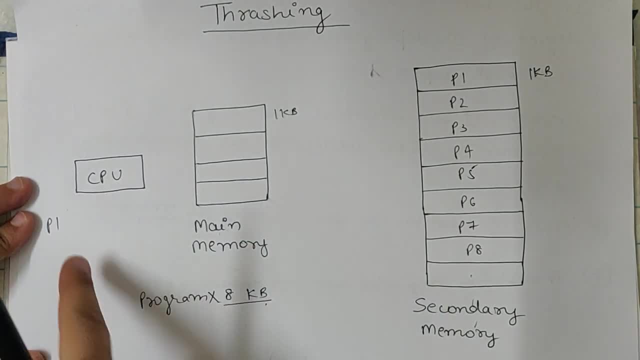 CPU demanded a page number 1.. Okay, page number 1, CPU will execute that. CPU will search that particular page inside the main memory, But P1 doesn't reside in the main memory. then page fault occurs And after the page fault occurs it will rest. So this is a 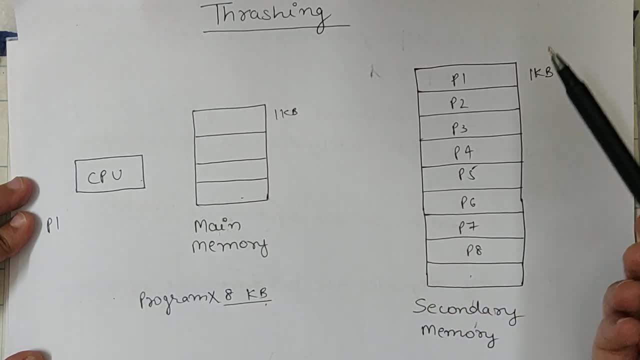 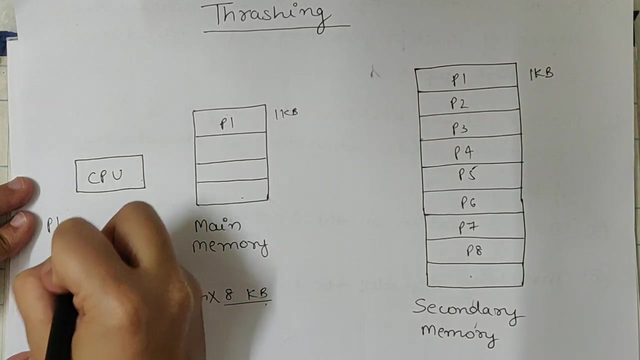 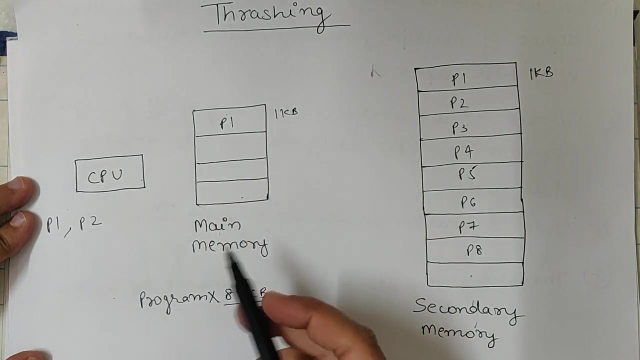 occurs, what will happen? operating system brings the p1 page from the secondary memory to the main memory and it will be now present in the main memory. so CPU picks up the p1 page and executed it. simple okay. now CPU demanded page number two again. CPU searches the main memory for p2 page, but p2 page is not present. 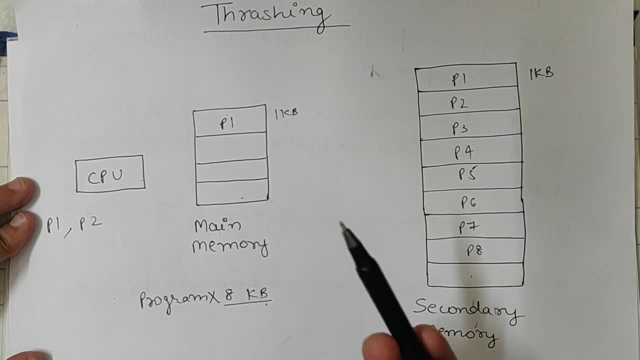 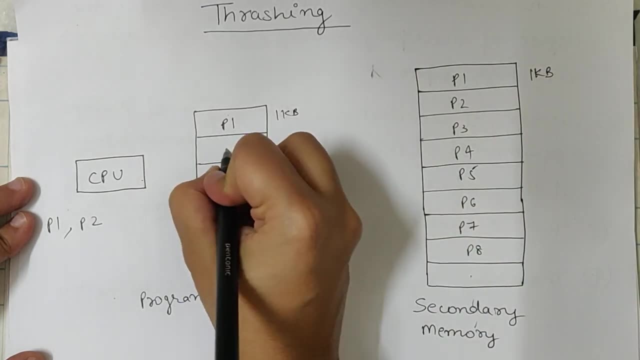 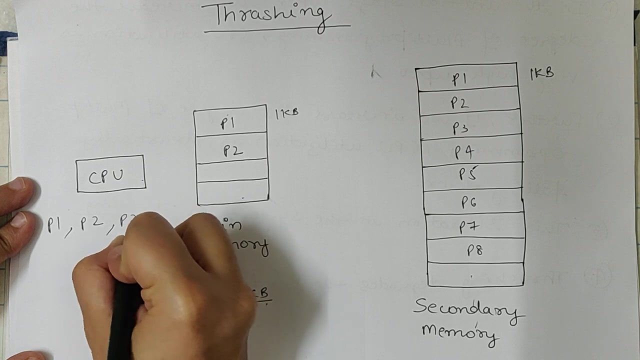 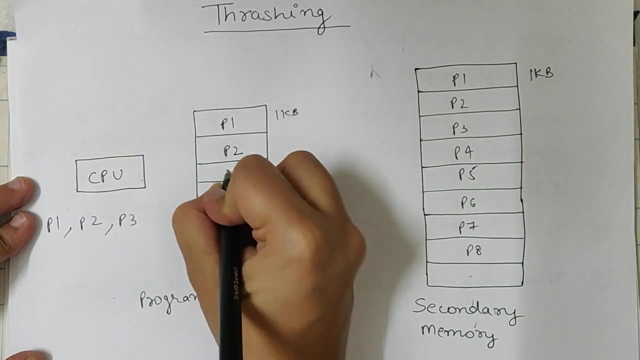 in the main memory. again page fault occurs. so now again operating system will bring back. bring the page number two to main memory. okay, now CPU will picks up the page number two and execute it. simple. now again CPU wants page number three. again page fault occurs. operating system: bring backs the p3 page. 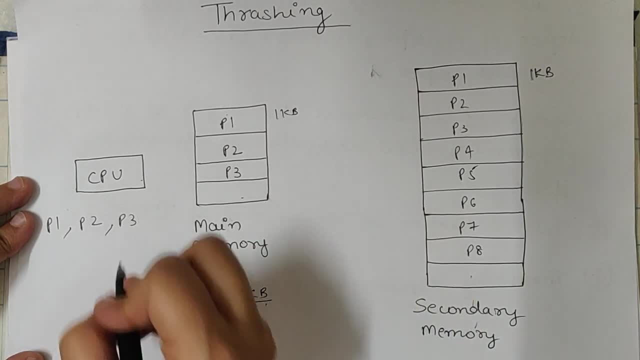 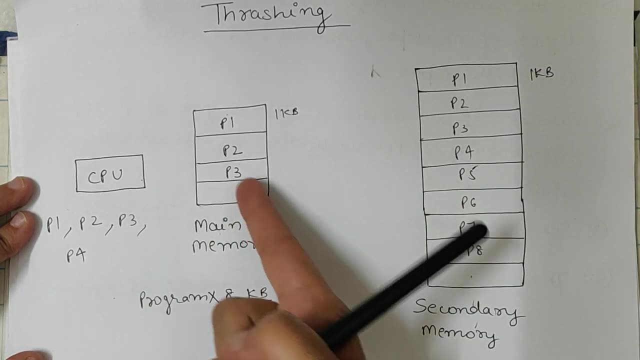 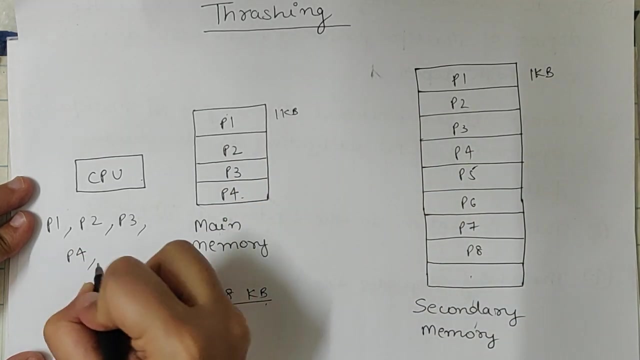 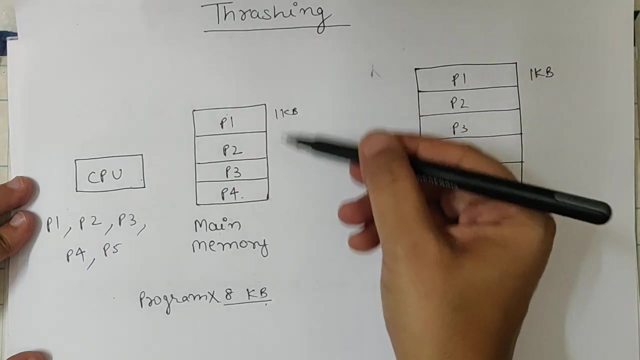 inside the main memory, from the secondary memory to main memory. okay, done. cp. now execute p3. now CPU wants page number 4. now it is also not present. so page fault occurs again. p4 we have taken from secondary memory to main memory. now CPU wants page number 5. CPU searches the page in main memory, but p5 is not. 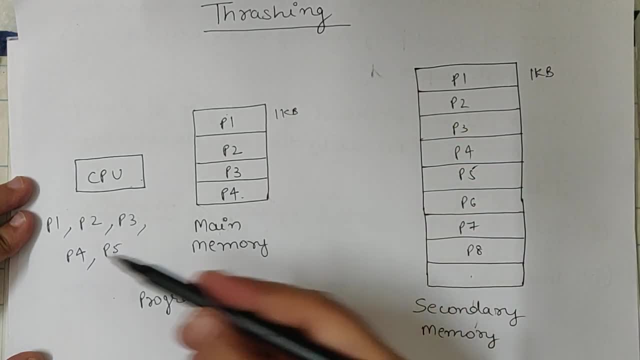 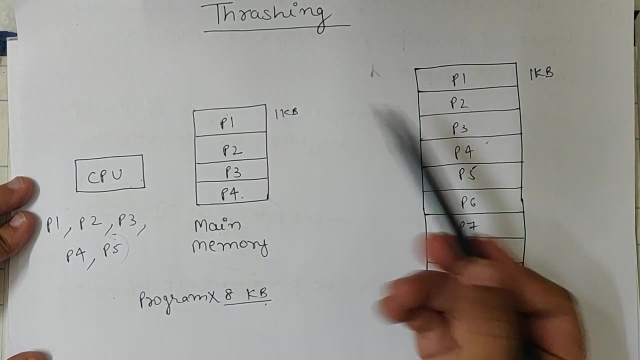 present in main memory. then page fault occurs. but CPU wants page number 5. we have to bring p5 inside the main memory. but main memory is full. so p1, p2, p3, p4 may say: kisi ko toh wapis se secondary memory mein jana padega na taaki space. 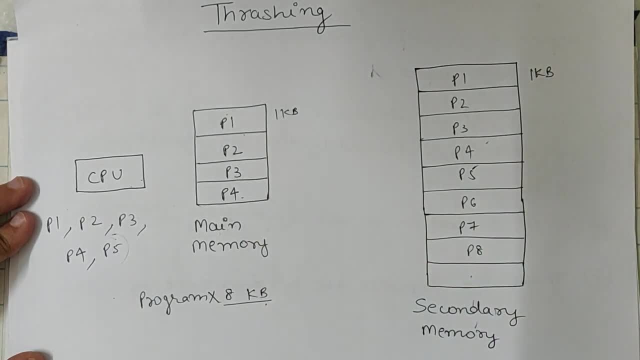 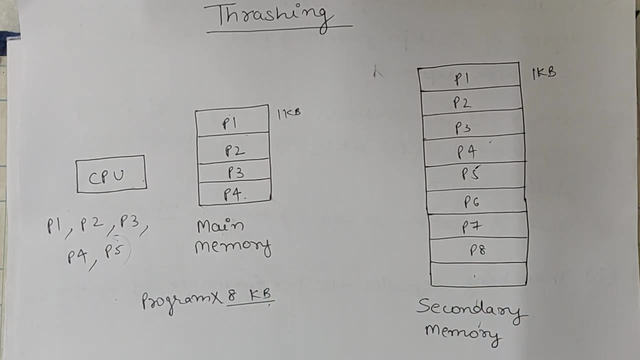 free frame ho jaye, aur p5 ki entry ho jaye toh kisi ko toh jana padega wapis backend store pe backing store pe jana padega secondary memory mein. toh thik hai, humne socha chalo p1 ko bhej dete hain. sabse pehle p1 hi aaya tha main. 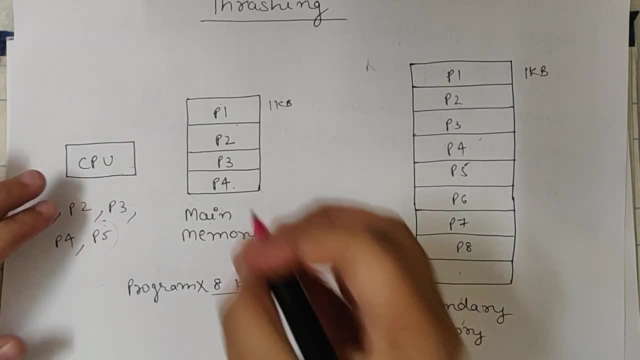 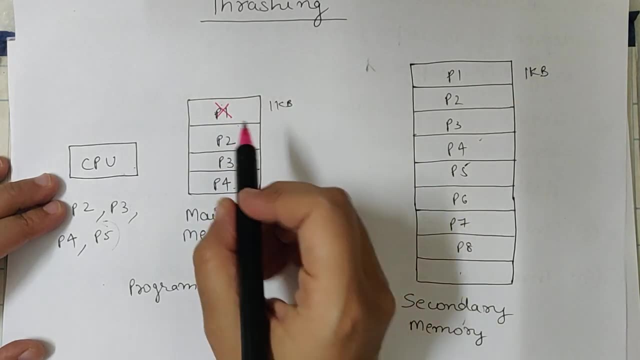 memory mein, toh we will bring back to p1. ko na humne bhej diya wapis secondary memory mein p1 chala gaya up free frame hai p5 ki entry ho sakte hai. na thik hai humne p5 ki entry. 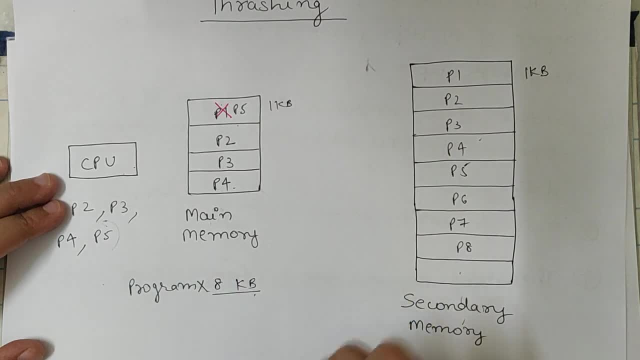 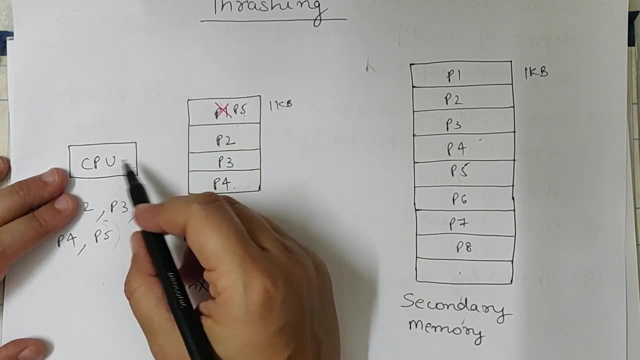 haan pe kardi p5 ki entry ho gayi. koi problem nahi hai, jaise hi p5 ki entry hoi na aur CPU p5 ko execute karne hi wala tha. abhi kara nahi tha execute, jaise hi p5 ki entry ho gayi main memory mein. now CPU will restart the. 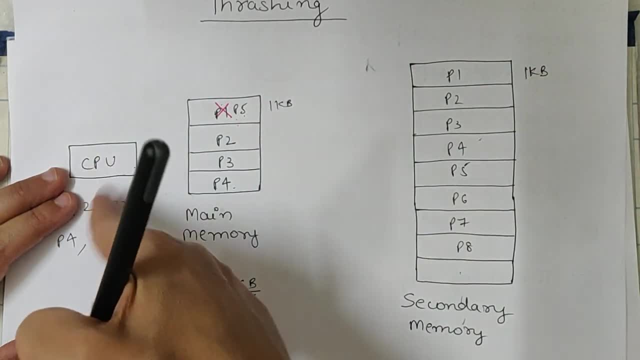 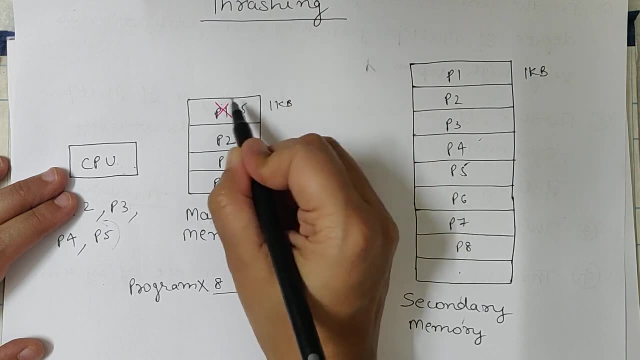 instruction wala maine jo bataya tha ja main memory, main memory, main memory main, main memory, main entry ho gayi uske baat. dubara jyab CPU nai search kiya aur p5 usko jase hi usko mila immediately usko p5 ke sath, sath p1 bhi. 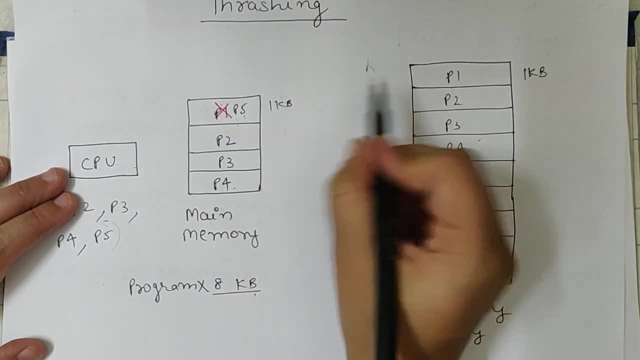 chahiye tha, jisko abhi abhi humne backend store pe beja. p5 bhi chahiye, aur p1 bhi chahiye. dona chahiye usko CPU ko jaise hi p5 ko humne main memory mein. 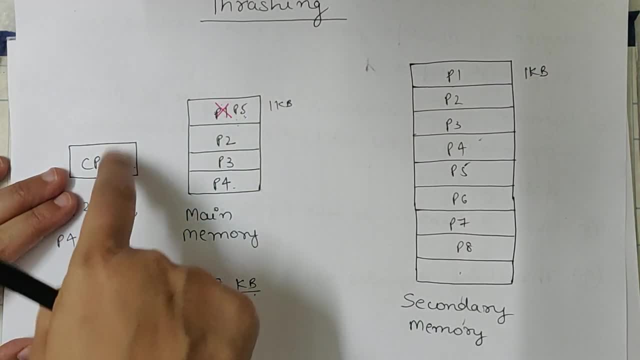 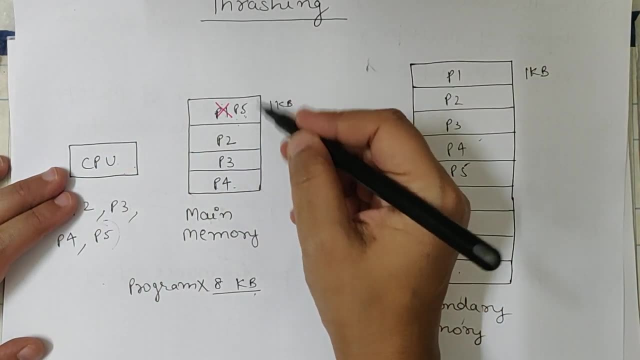 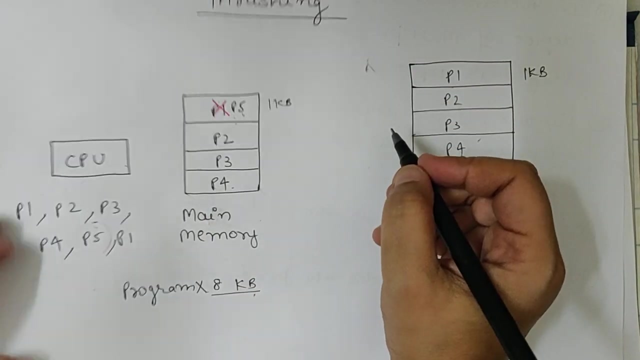 load kiya execute karne se pehle CPU p5 ko execute karne hi wala tha ki immediately usko p1 ki dubara requirement pad gayi, but ab firse main memory full CPU demanded P1, so we have to bring P1 back from back-end store. 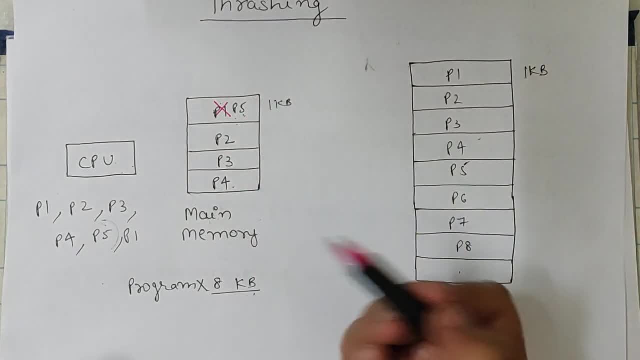 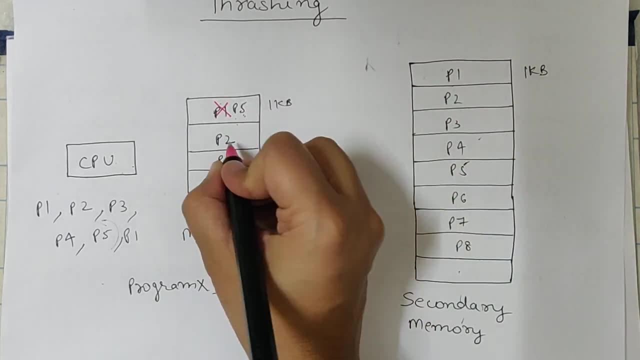 Now we thought of sending P2, because main memory is full, so we have to bring P1.. If we don't bring P1, then P5 will not be executed. So we sent P2 back to back-end store and we brought P1 back here. 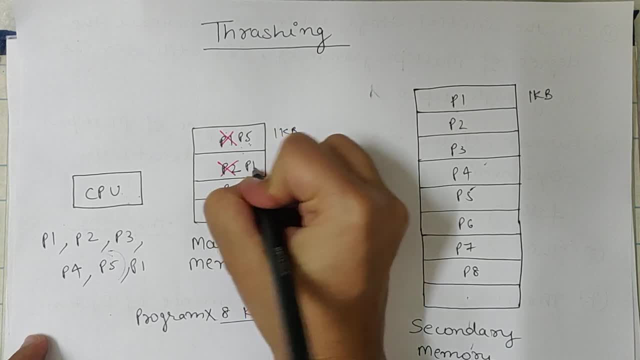 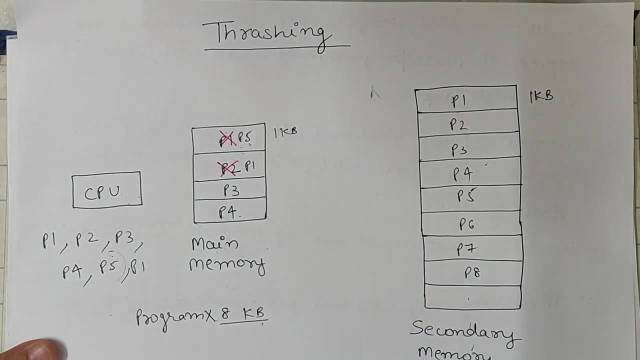 We brought P1 back here Now CPU was about to execute P5 and P1, but it got P2 requirement. We just sent P2 back to back-end store But CPU said I want page number 2, otherwise it will not be able to execute P1 and P5. 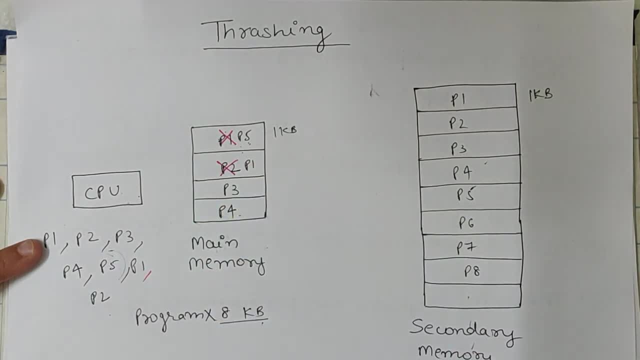 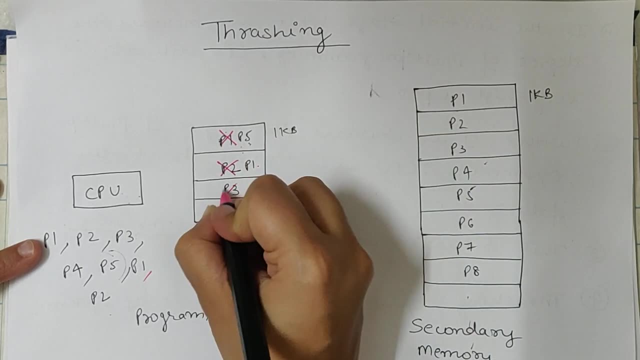 CPU wants P2 page. so we thought we can't send P3 back to back-end store because CPU requires P5 and P1 as well as P2.. So we thought of sending P3 back to back-end store. So we thought of sending P3 back to back-end store and we brought P2 back to back-end store. 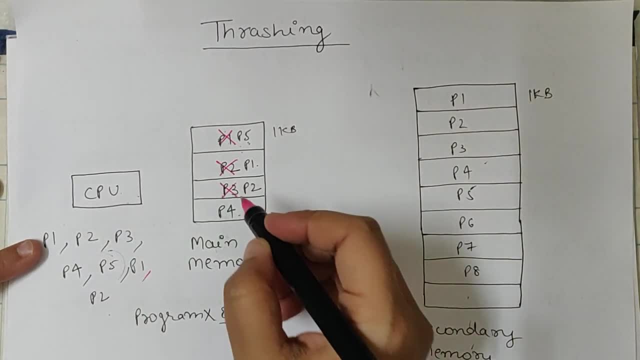 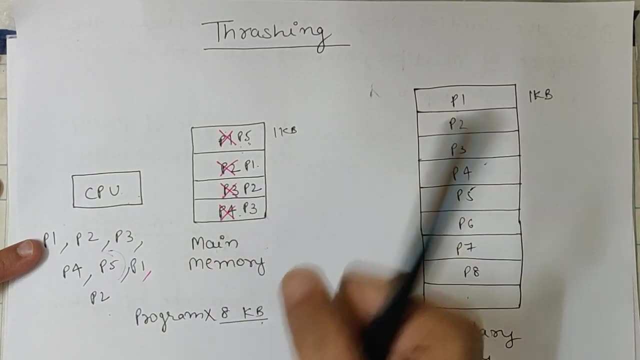 As soon as we brought P2 back to back-end store. now we don't want, CPU wants, we want page number 3.. So we removed P4 and added P3.. Now CPU wants: no, I want P4 also. So what are we doing? We are not executing anything. 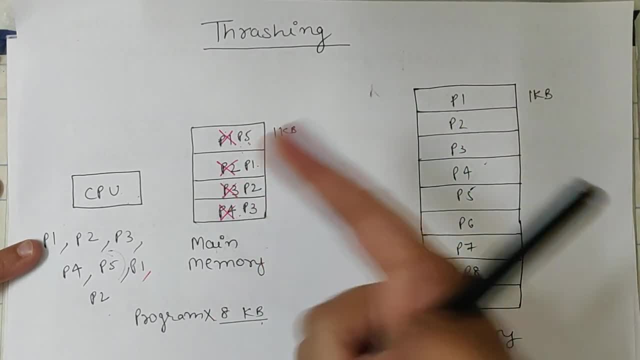 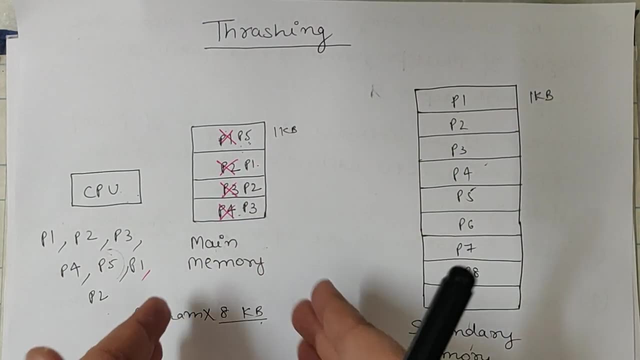 What we are doing is swapping- swap in, swap out, swap in, swap out- Or we are just paging. Keep it as we are. We are doing the same thing. We are putting the page in the main memory from secondary memory. 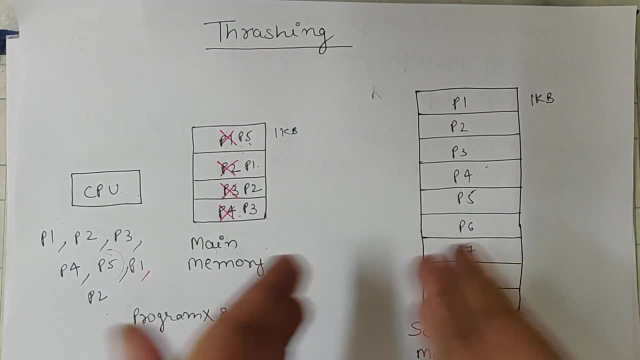 As soon as we send that page in the secondary memory, we immediately put it in the main memory, Then we send it to the main memory. So the CPU is not executing anything for this long. So just swapping and swap out. This is what we are doing. 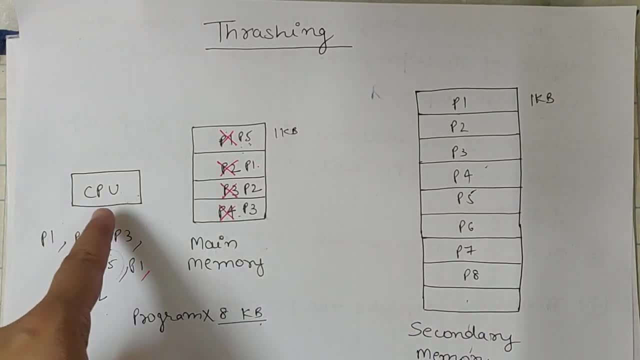 We are paging. whatever we are doing, We are not utilising the CPU properly. We are not utilising CPU in any way. We are only unload-load and load the pages in the main memory. Swap in swap out only we are doing. 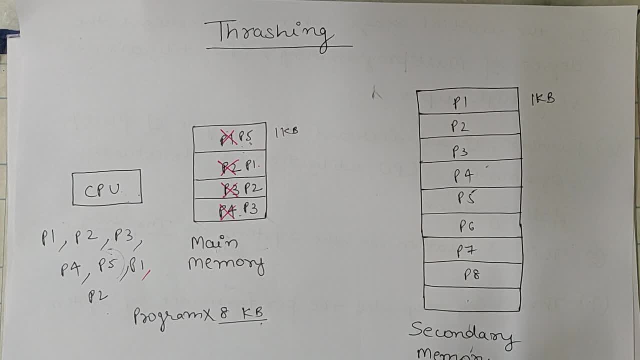 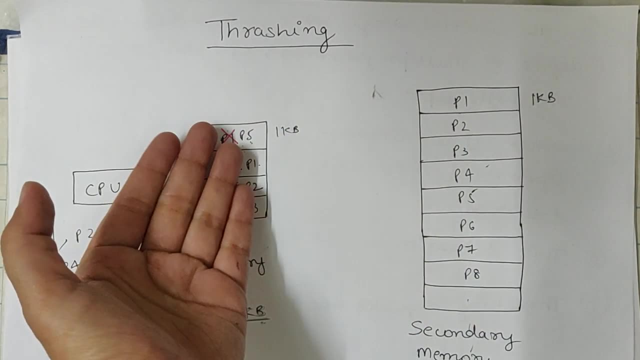 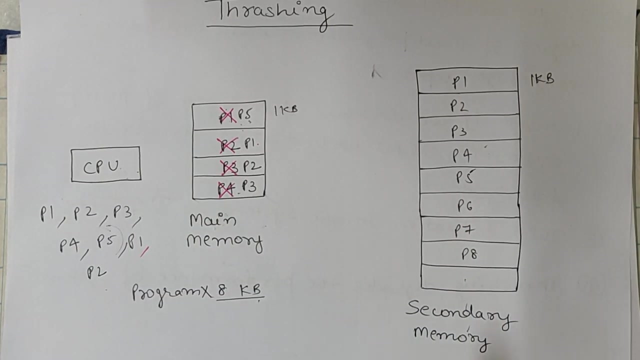 So this is a problem, that our time is not going in execution. what we are doing is that whichever page we bring, whichever page we leave in secondary memory, we demand the same page's CPU again. So CPU is not executing in execution, it is not executing anything. it is doing paging. 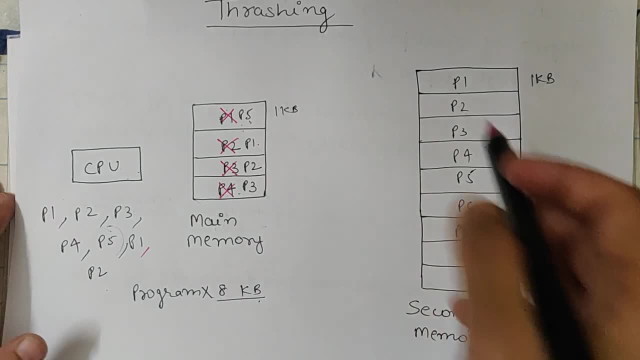 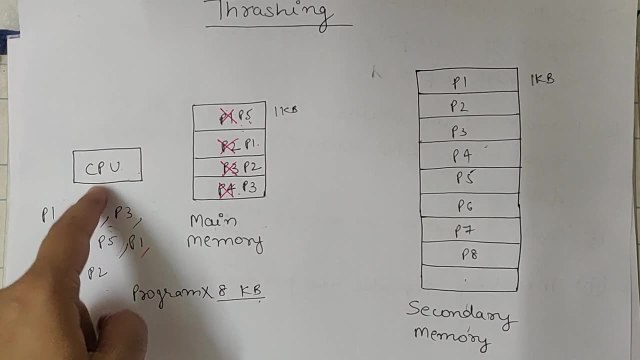 activity. again and again it is doing swap in, swap out, and this problem is known as threshing. We call high paging activity as threshing When CPU's main memory gets full, when it comes to replacing the page as soon as we 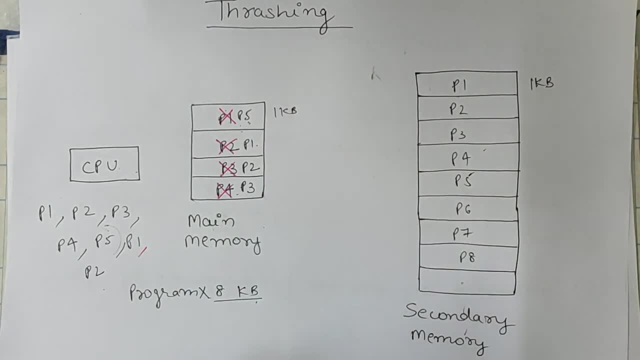 replace the particular page, immediately the requirement of that page gets read to CPU and then, as soon as we bring that page again, the requirement of the one who is replaced gets read. Like in our case: if we send P1, P5 comes, then CPU wants that, I want P1, we keep P1. 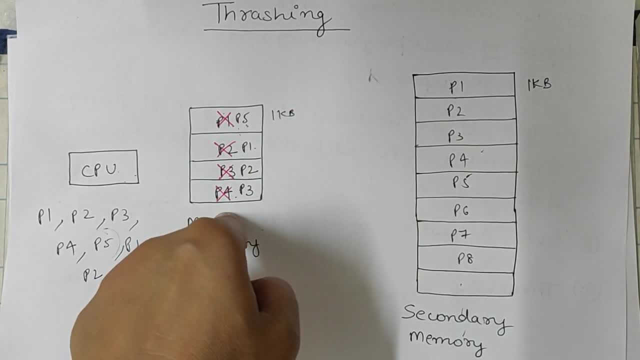 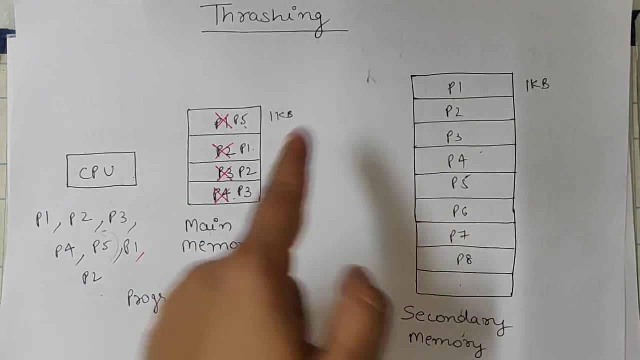 then we want P2, we send P2 back and P3, we send P3 back, we keep P2, then we say: we want P3,, we want P3, we send P4 back. then we get P3, you are saying: we want P4. 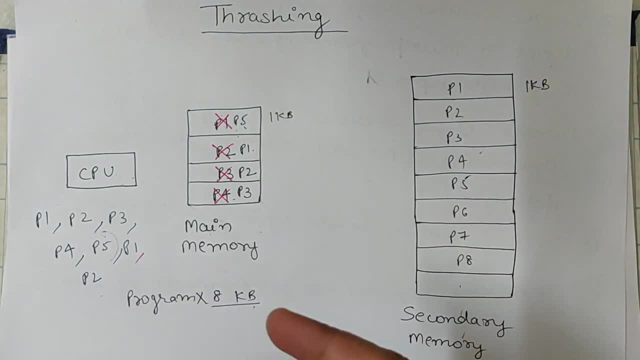 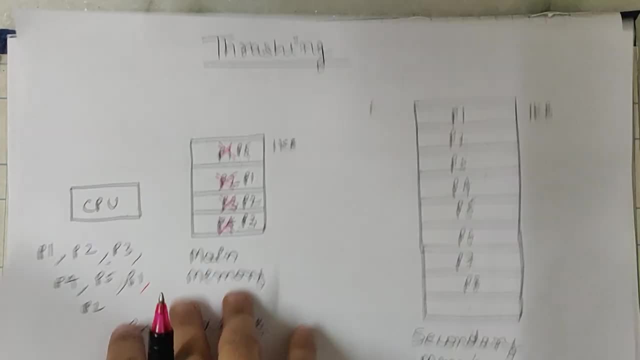 Again, if we remove P5, then we say we want P5,, we also want P4. So this problem is known as threshing Clear. These are some points. you can go through this whole In the initial stage when we increase. 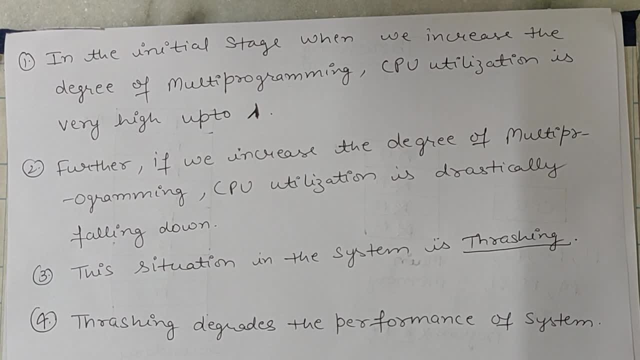 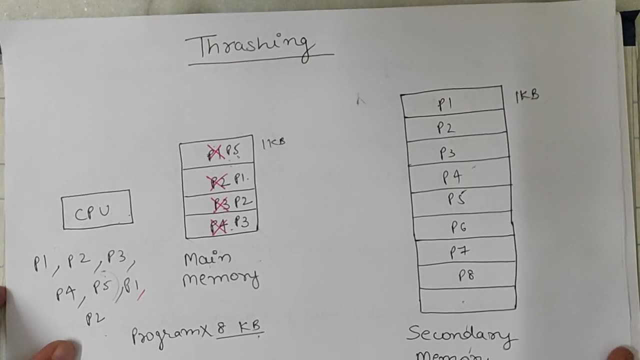 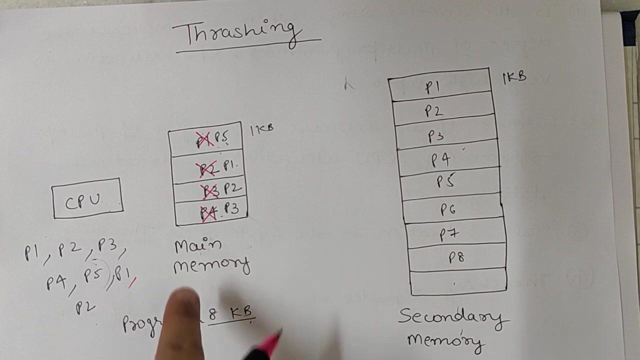 The degree of multi-programming CPU utilization is very high, up to lambda. Okay, What does this mean? I will explain it with this diagram: only Degree of multi-programming. What does multi-programming mean When we have pages loaded in main memory? 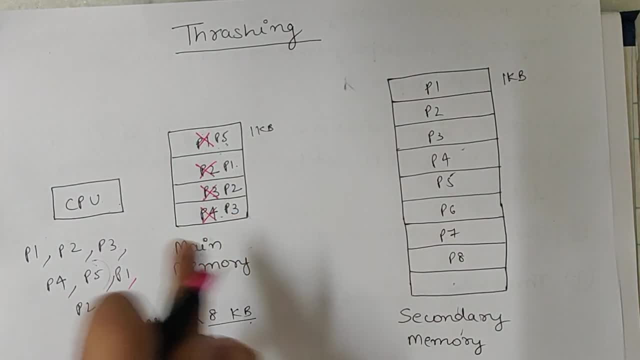 Okay, When many programs are loaded in main memory, that is called multi-programming. So it is saying that initially what happened. Main memory is empty, so P1 got loaded. Okay, Page fault happened, but we brought the page from secondary memory to main memory. 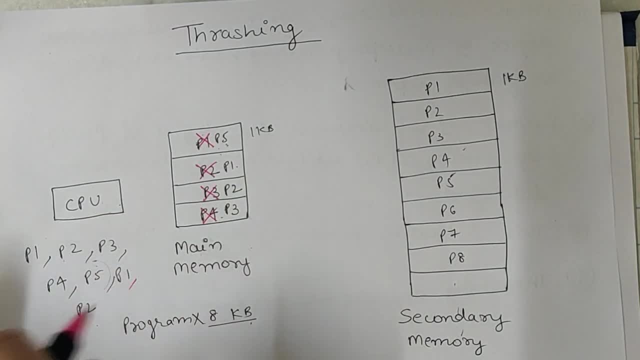 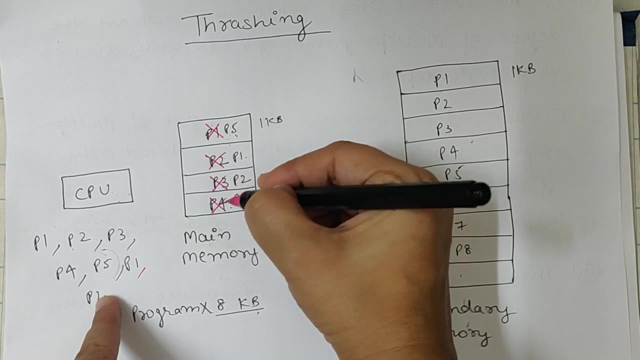 So CPU had executed the page. So CPU utilization was initially very good when multi-programming degree was increasing Means. as soon as P1, P2, P3, P4 were coming line by line, then CPU was executing. 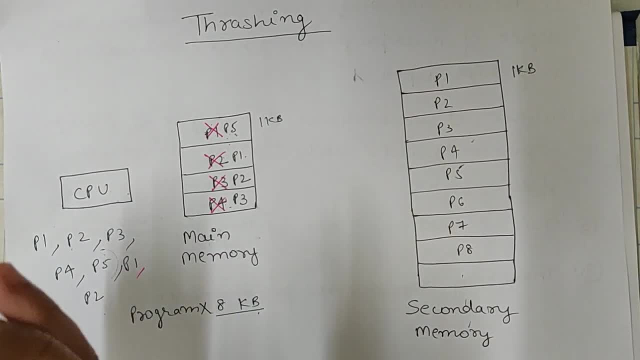 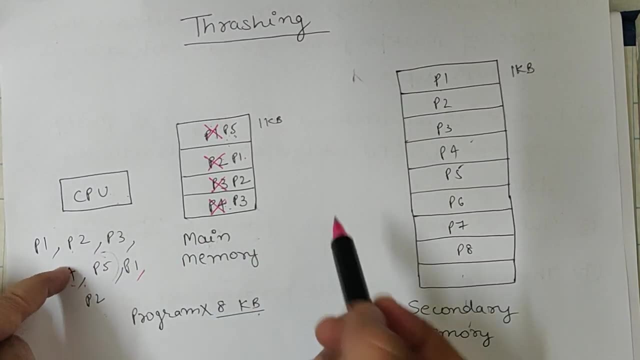 So initially it was going very well up to lambda. Lambda means as soon as P1, P2, P3, P4, our work was going very well. But as soon as it was time to replace, At that time there was a downfall. 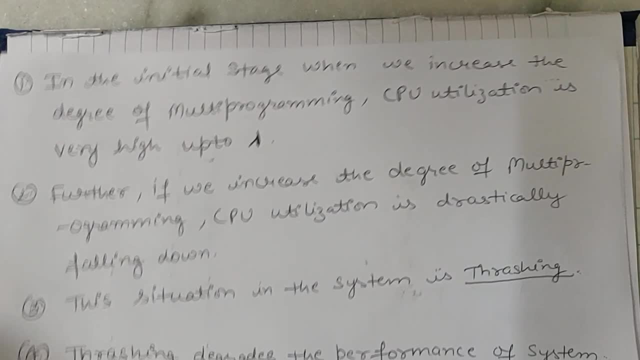 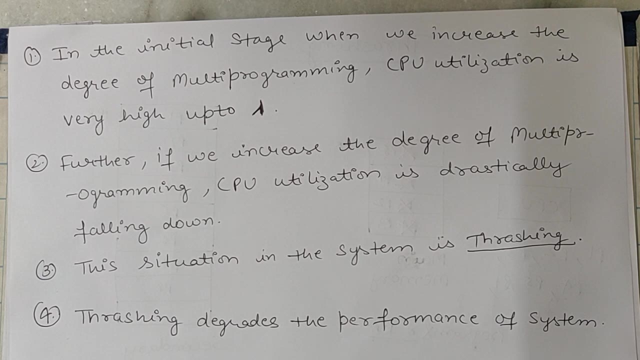 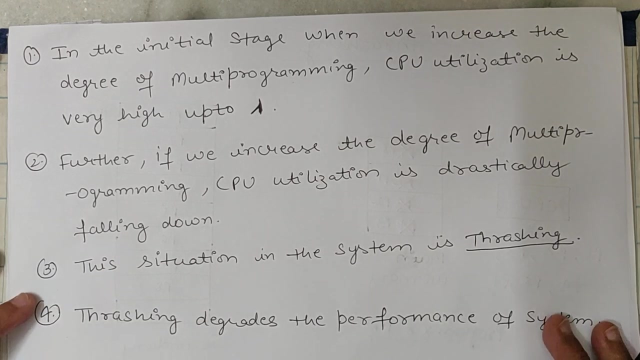 Okay. So it is saying that initially, when we increase the degree of multi-programming, Means when we were putting P1, P2, P3, P4, till then CPU utilization is very high, up to lambda. But further, if we increase the degree of multi-programming, CPU utilization is drastically falling down. 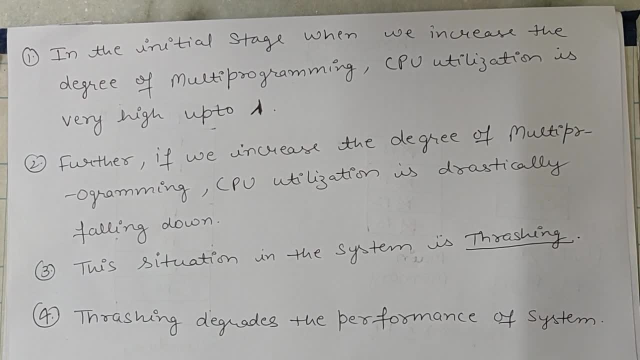 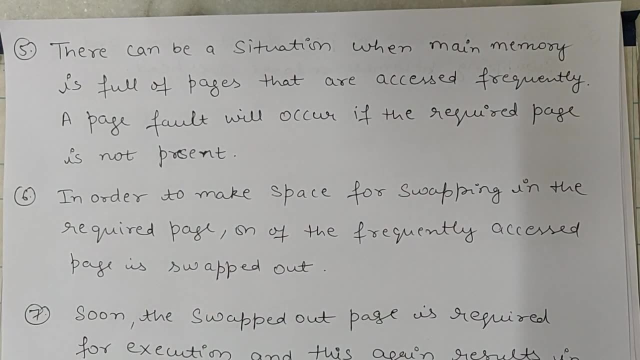 And this situation in the system is called thrashing. Thrashing degrades the performance of the system. Okay, Fifth point is there can be a situation when main memory is full of pages that are accessed frequently. A page fault will occur if the required page is not present. 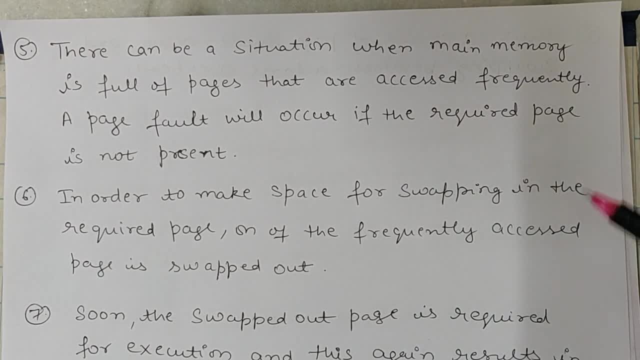 Okay, So I have already explained all this to you. Okay, In order to make space for swapping in the required page, one of the frequently accessed pages is swapped out. Okay, This is what we did: Swap in, swap out. 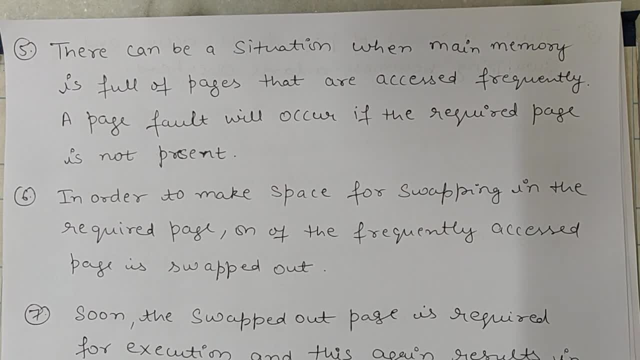 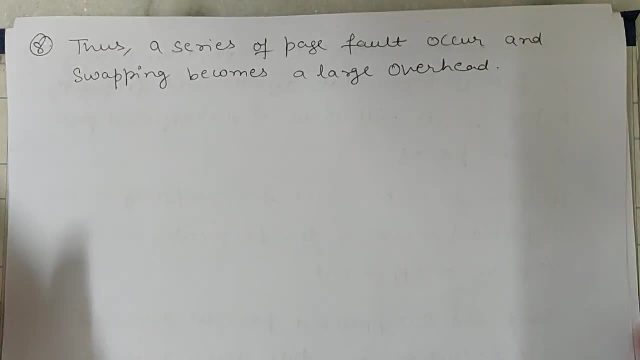 Okay, Swap out. Soon. the swapped out page is required for execution and this again results in page fault. Okay. Thus a series of page faults occur and swapping becomes a large overhead. These are some points related to thrashing Okay. 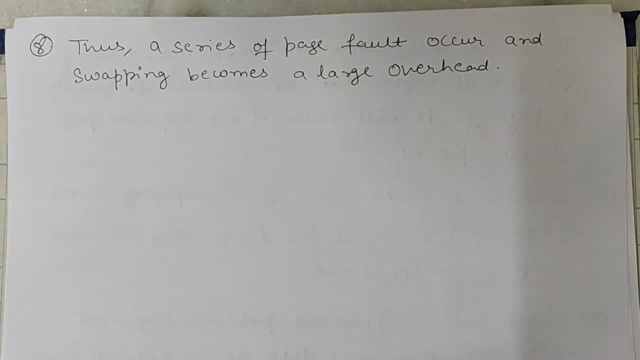 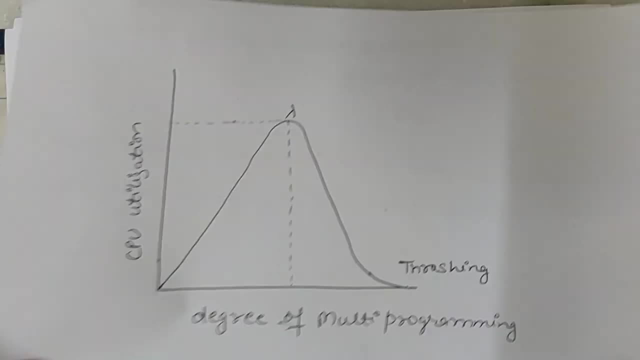 As soon as we send the page of swap out, then there is a requirement of the swapped out page. So we are doing the paging activity again and again. That is known as thrashing. So this is the very important diagram, A very important graph related to thrashing. 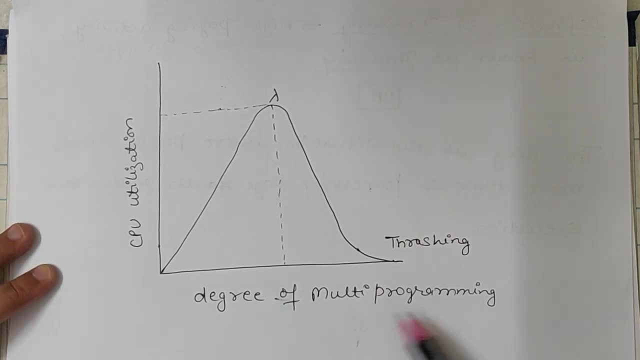 This is a very important graph of thrashing. Here on the x-axis there is a degree of multi-programming. That means page 1 is coming, page 2 is coming, page 3, page 4.. This is the degree of multi-programming of the pages that are coming in the main memory.